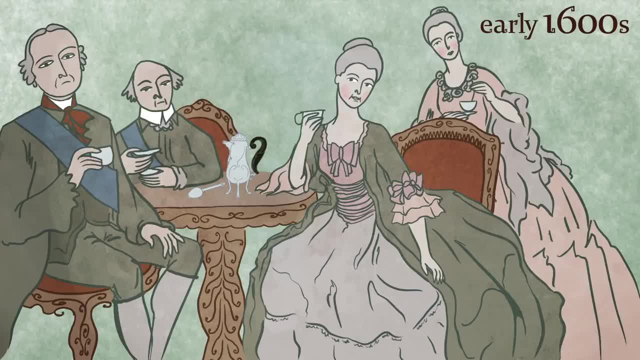 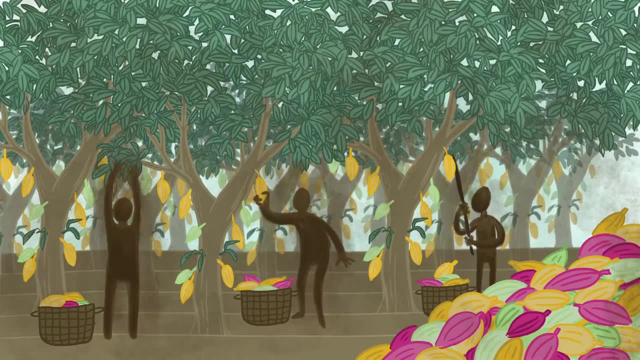 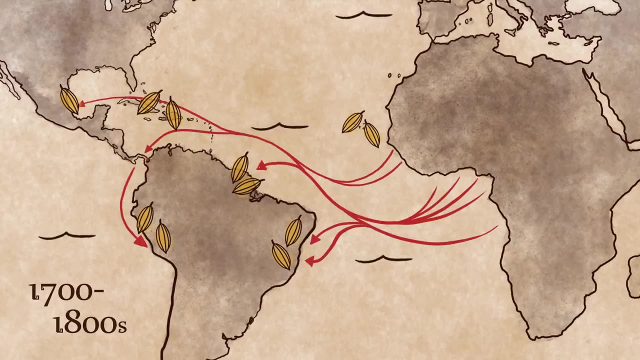 And soon. no aristocratic home was complete without dedicated chocolate ware. The fashionable drink was difficult and time-consuming to produce on a large scale. That involved using plantations and imported slave labor in the Caribbean and on islands off the coast of Africa. 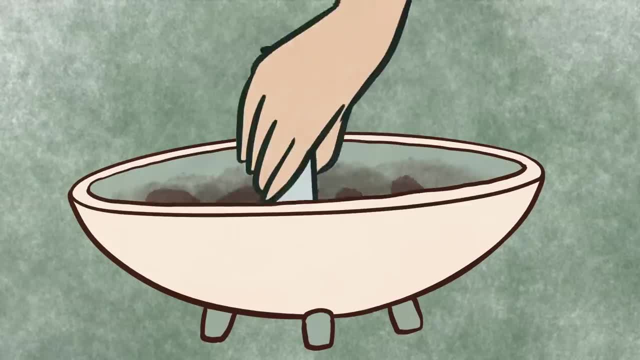 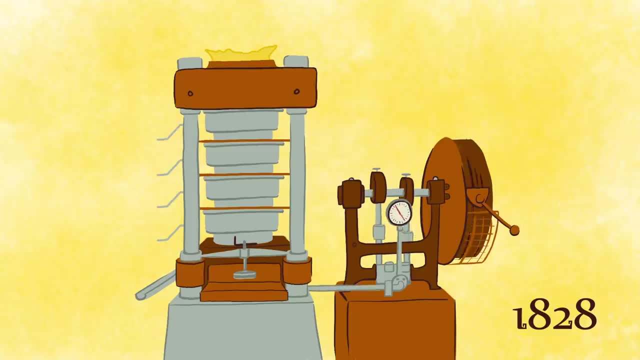 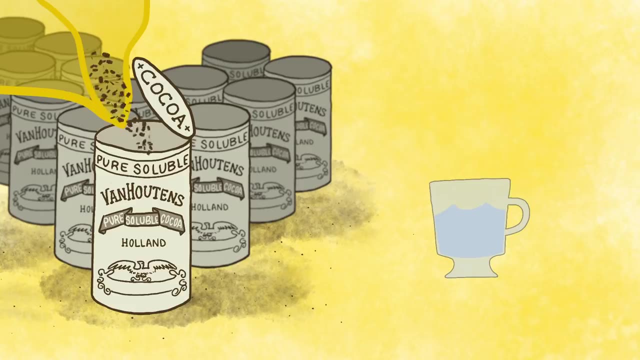 The world of chocolate would change forever in 1828, with the introduction of the cocoa press by Conrad Van Houten of Amsterdam. Van Houten's invention could separate the cocoa's natural fat or cocoa butter. This left a powder that could be mixed into a drinkable solution. 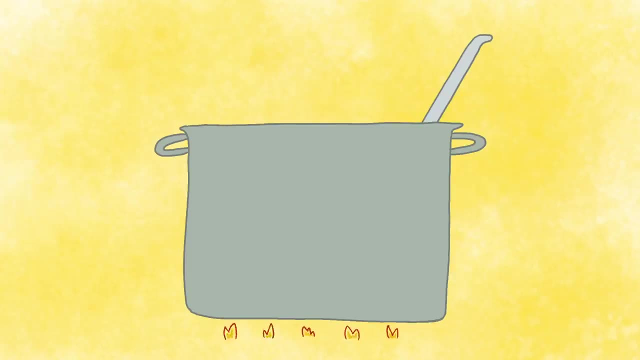 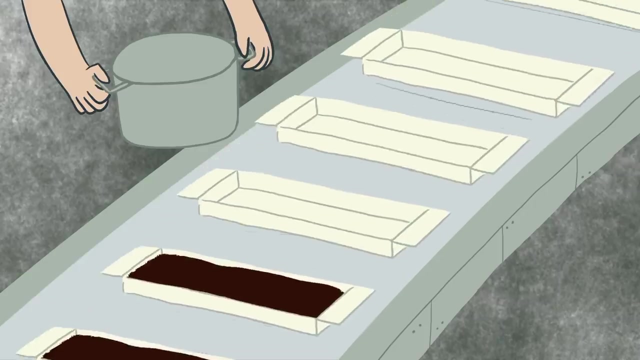 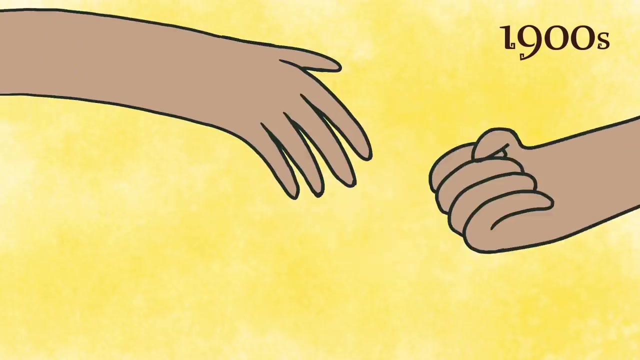 or recombined with the cocoa butter to create the solid chocolate we know today. Not long after, a Swiss chocolatier named Daniel Peter added powdered milk to the mix, thus inventing milk chocolate. By the 20th century, chocolate was no longer an elite luxury. 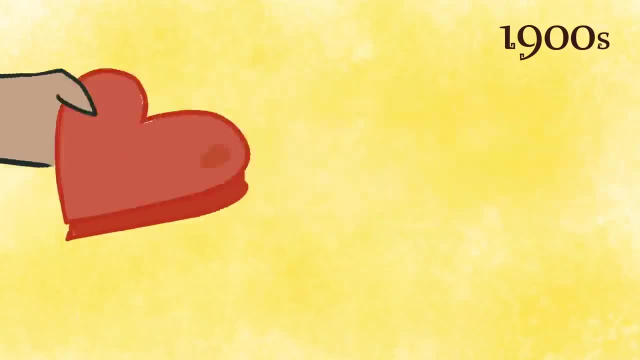 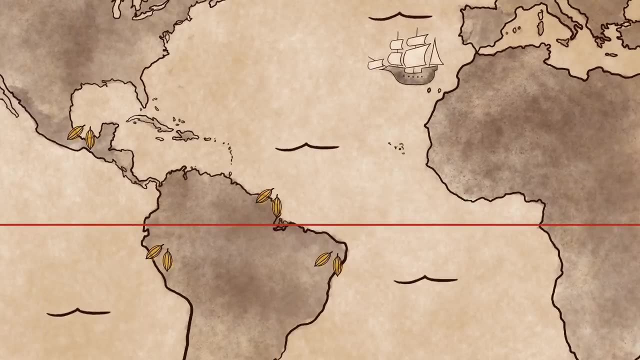 but had become a treat for the public. Meeting the massive demand required more cultivation of cocoa, which can only grow near the equator. Now, instead of African slaves being shipped to South American cocoa plantations, cocoa production itself would shift to West Africa. 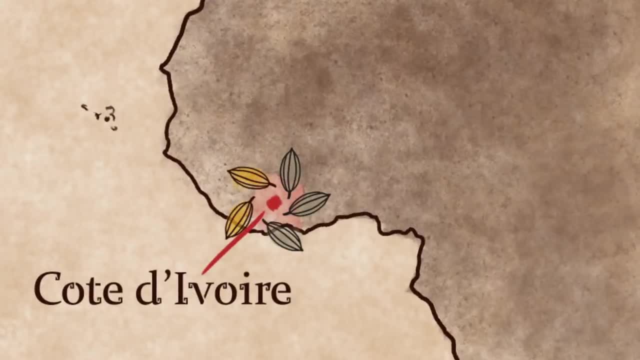 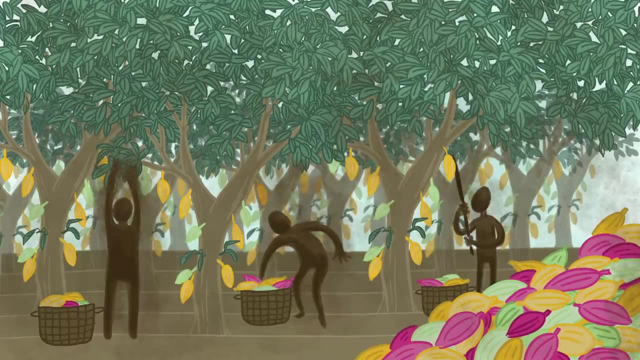 with Côte d'Ivoire, providing two-fifths of the world's cocoa as of 2015.. Yet, along with the growth of the industry, there have been horrific abuses of human rights, Many of the plantations throughout West Africa which supply Western companies. 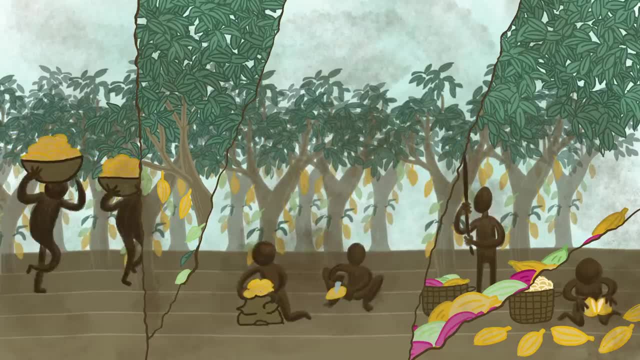 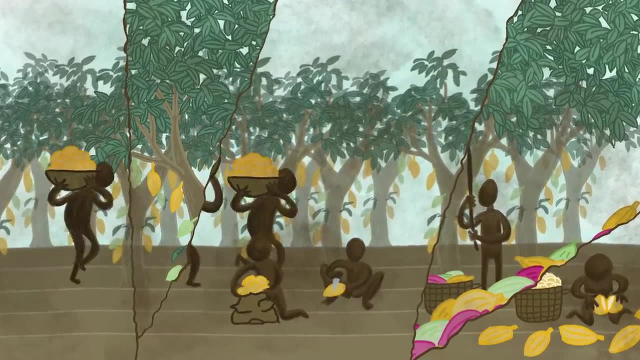 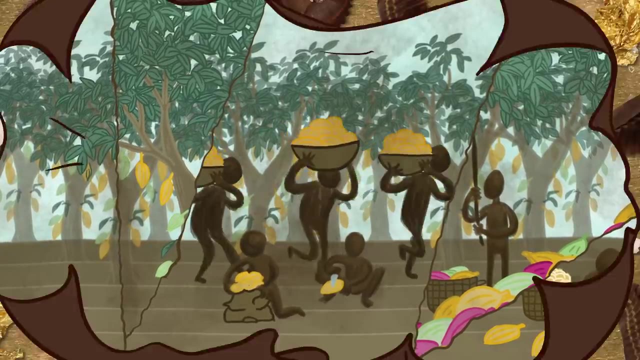 use slave and child labor, with an estimation of an estimation of more than two million children affected. This is a complex problem that persists despite efforts from major chocolate companies to partner with African nations to reduce child and indentured labor practices. Today, 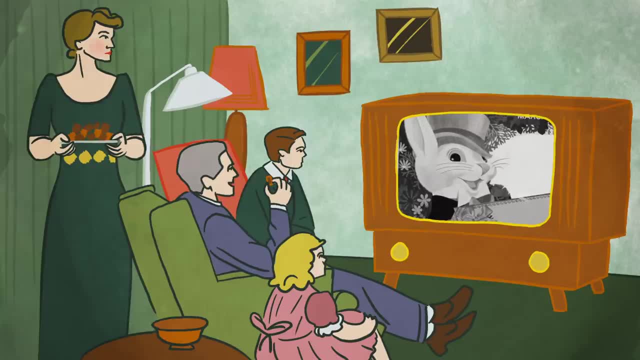 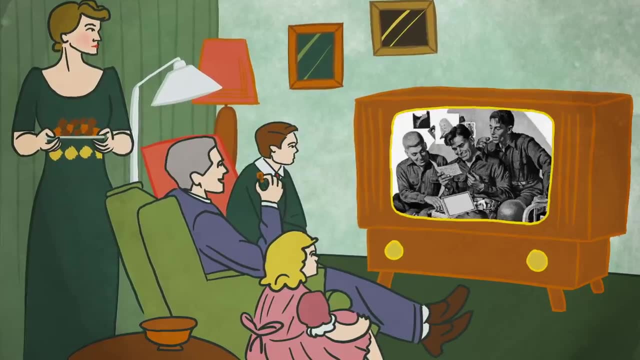 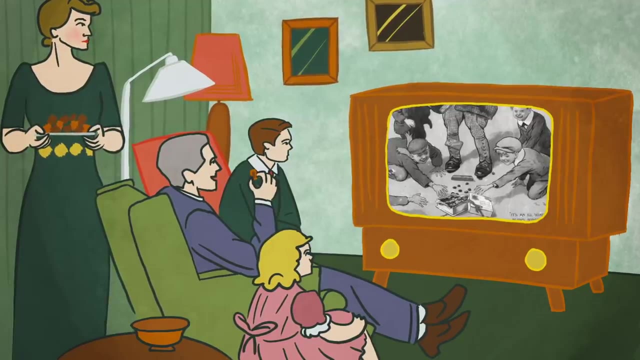 chocolate has established itself in the rituals of our modern culture Due to its colonial association with native cultures. combined with the power of advertising, chocolate retains an aura of something sensual, decadent and forbidden, Yet knowing more about its fascinating and often cruel history, 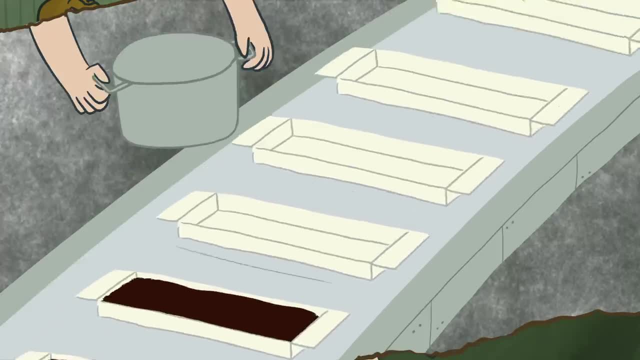 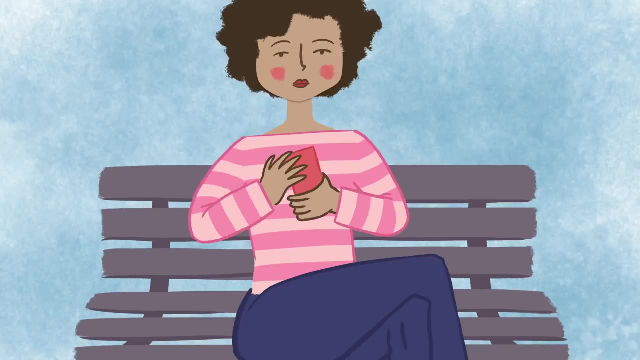 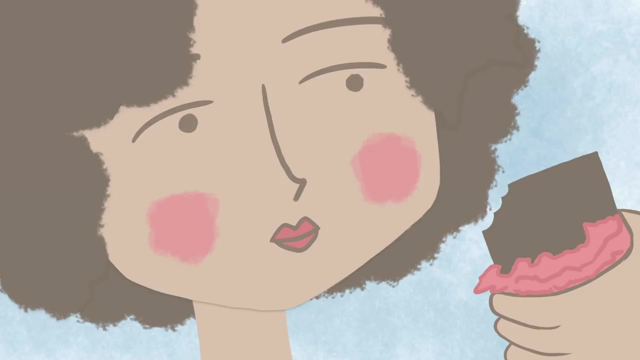 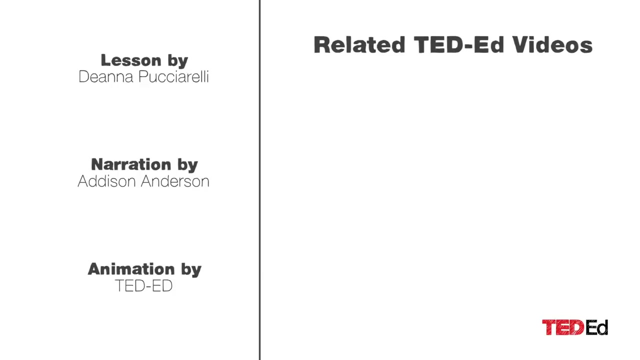 as well as its production, today tells us where these associations originate and what they hide. So, as you unwrap your next bar of chocolate, take a moment to consider that not everything about chocolate is sweet. If you want to learn more about chocolate,